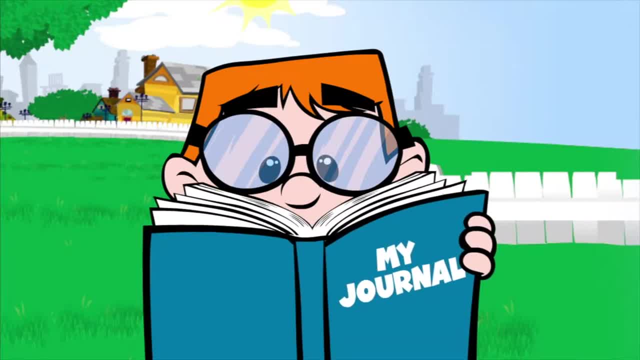 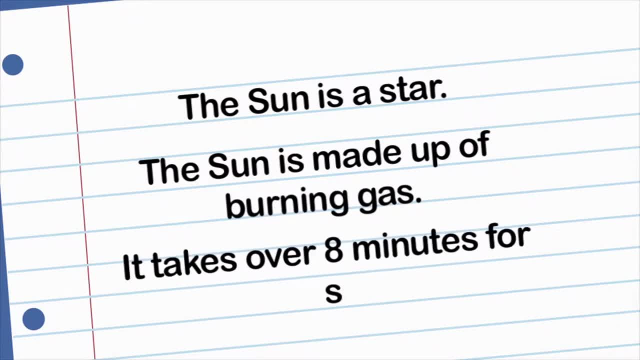 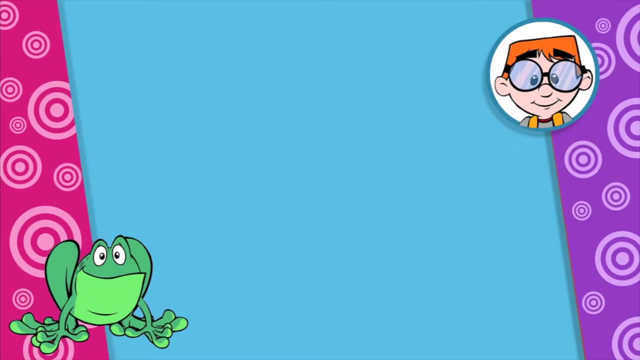 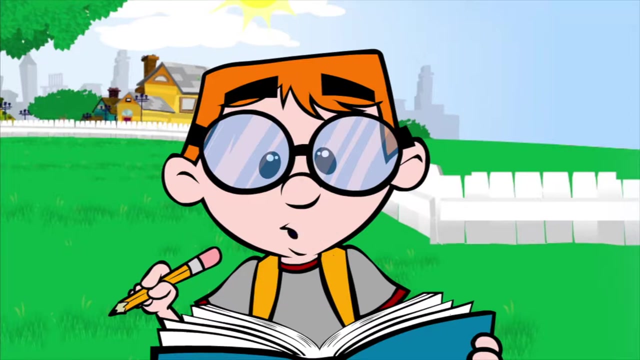 I'm going to write that down in my journal. So the sun is a star. It's made up of burning gas and it takes sunlight over eight minutes to travel to Earth. Got it The sun and the seasons. The sun heats the earth, but why is it hot in the summer and cold in the winter? 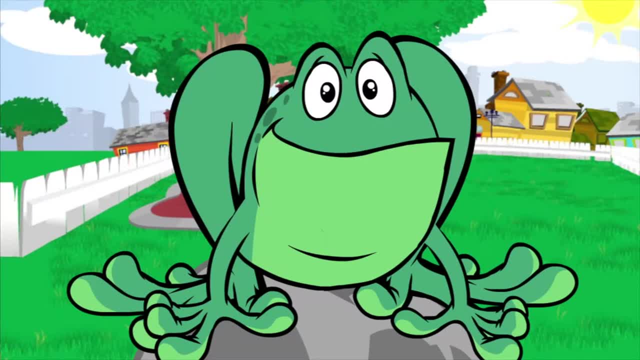 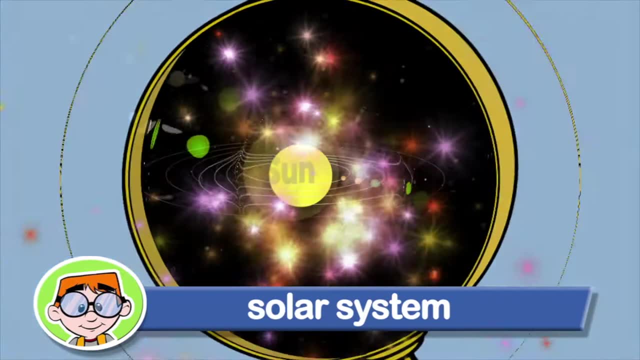 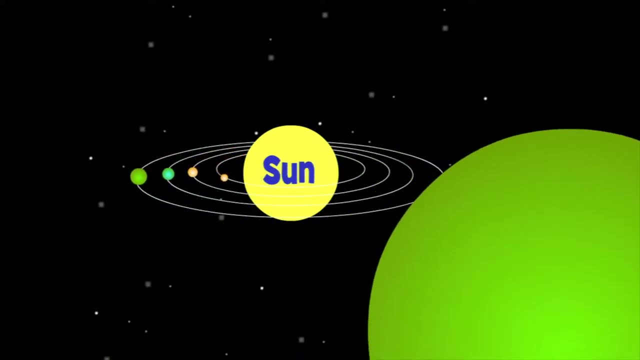 I was wondering the same thing. Excellent question. To best understand, we have to take a look at our solar system. The sun is part of our solar system. The earth and seven other planets and moons, comets, asteroids, dust and gas move around the sun. 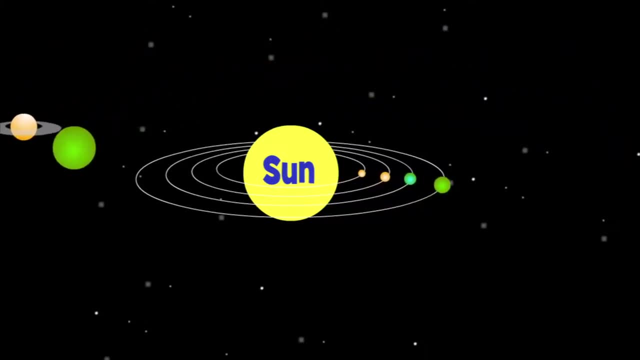 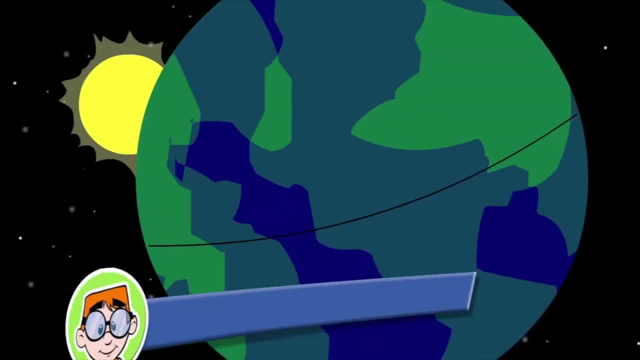 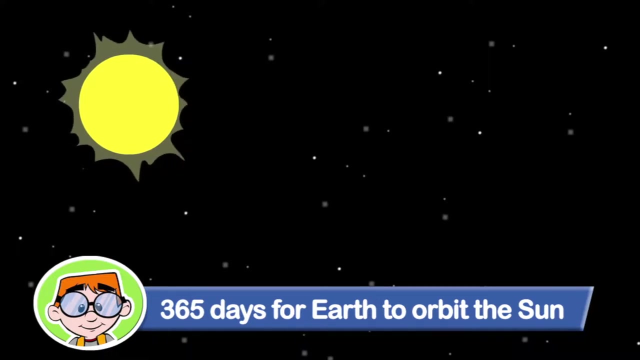 And the sun is the largest object in our solar system. Just like everything else in our solar system, Just like everything else in our solar system, Just like everything else in our solar system, The earth travels or orbits around the sun. It takes the earth 365 days, or one whole year, to orbit one time around the sun. 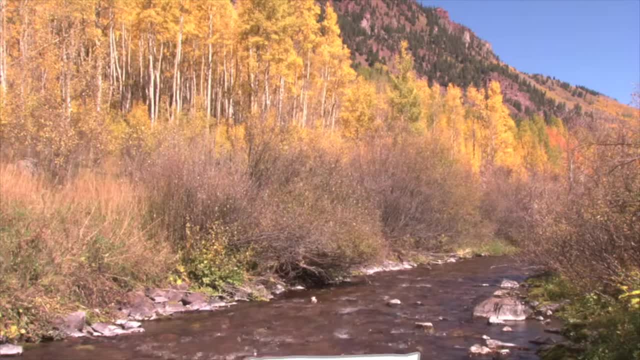 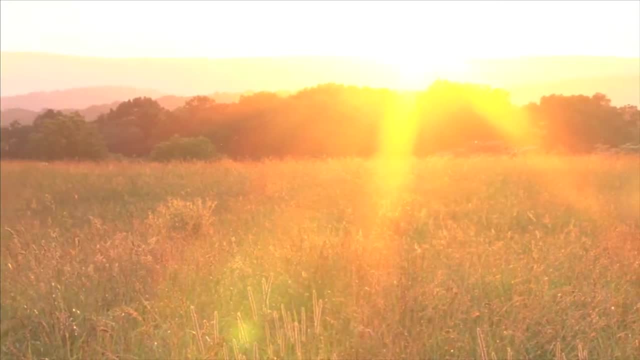 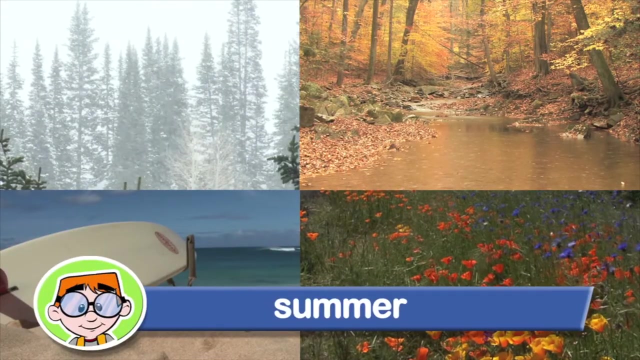 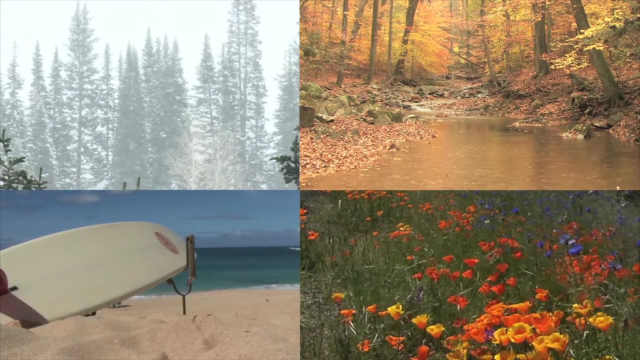 In that one year, the seasons and the weather change many times. The sun controls the weather and four seasons on earth. The four seasons are summer, spring, winter and fall. To understand how it works, you have to know a little bit more about the earth. 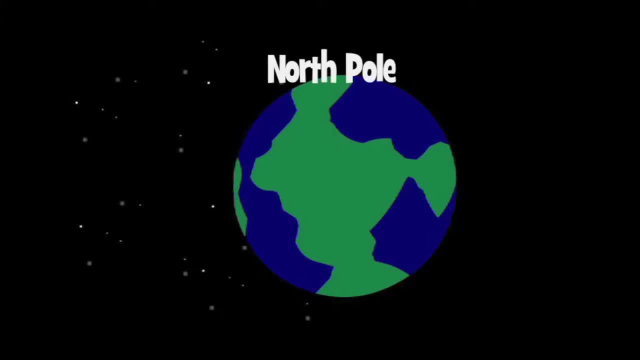 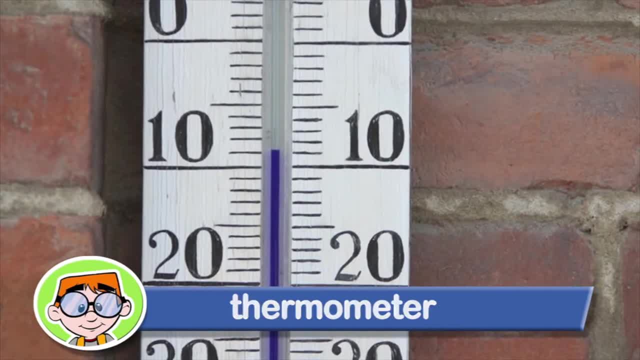 There is an imaginary line called the axis that goes from the north pole through the earth to the south pole, through the earth to the south pole. but of courseitung cannot rank some other number, as though its similar to 0. People use thermometer to measure temperature. 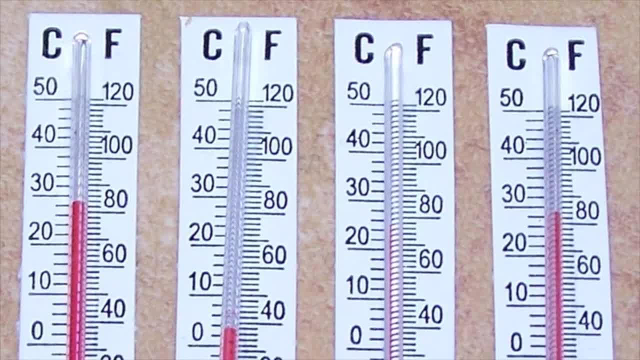 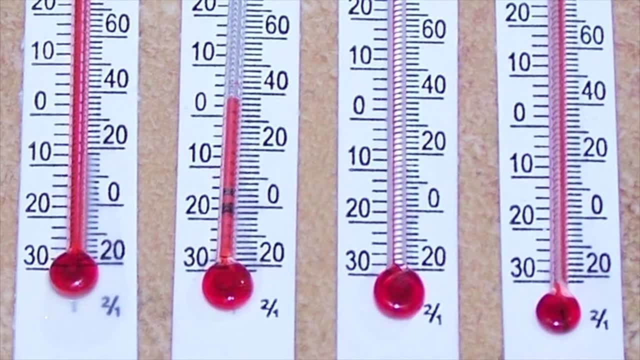 People use thermometer to measure temperature. Temperature is measured in degrees. Temperature is measured in degrees. An old fashioned thermometer uses liquid- mercury or another kind of liquid in a glass tube with a bulb at the bottom, or another kind of liquid in a glass tube with a bulb at the bottom. 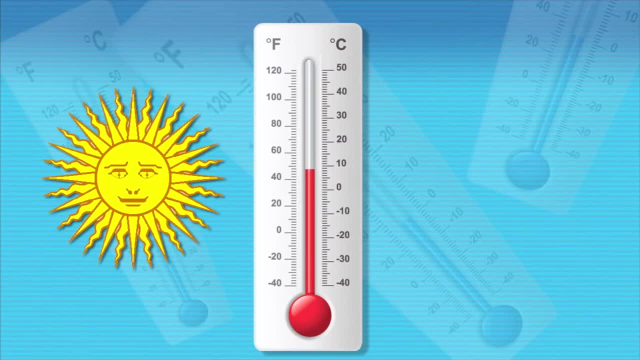 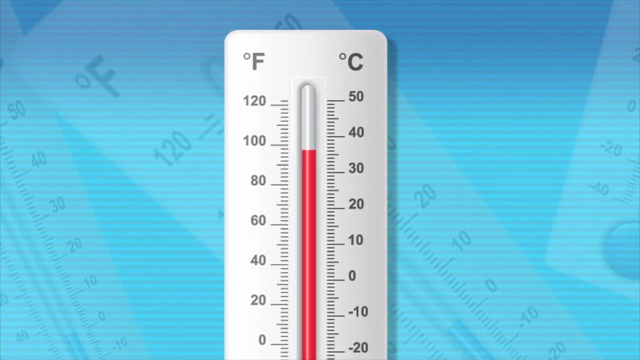 As it gets hotter, the liquid heats up. The molecules in the liquid begin to move and take up more space. As it gets hotter, the liquid heats up. liquid moves up the tube. The numbers on the side of the tube are used to measure how far up the liquid rises. People use different scales to measure temperature. 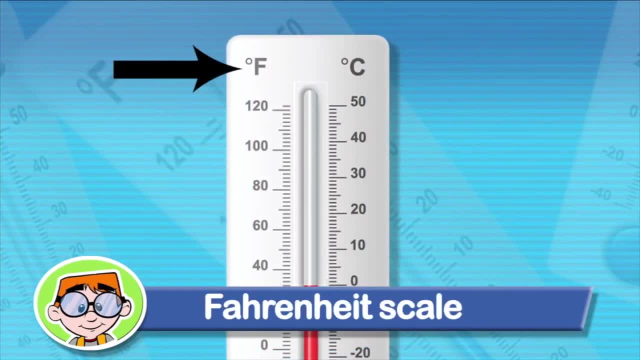 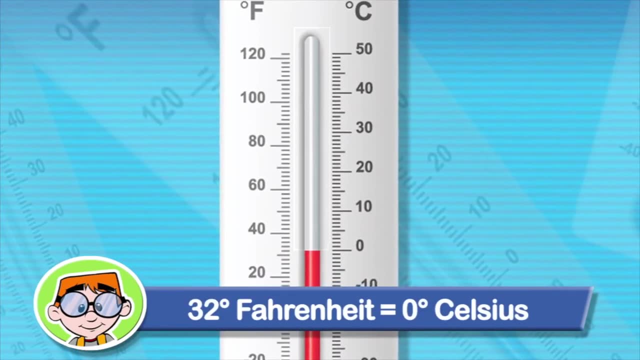 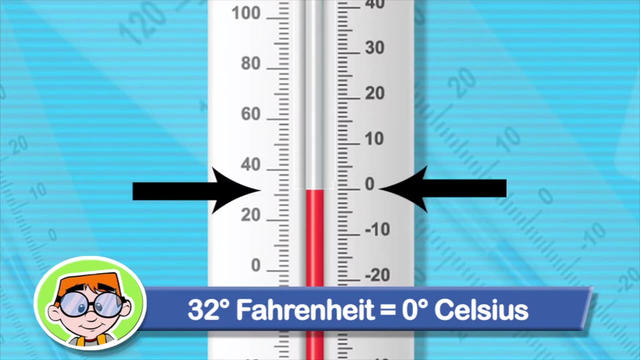 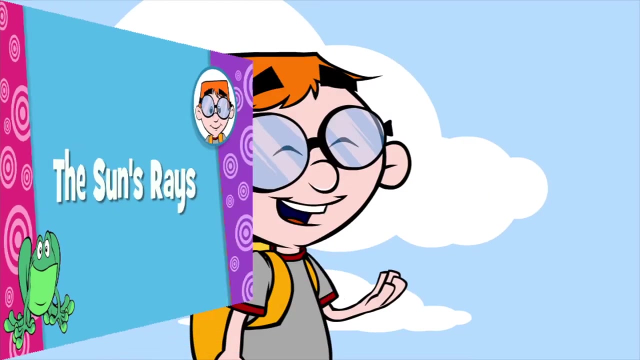 This thermometer measures on Fahrenheit scale and the Celsius scale. You'll see that 32 degrees Fahrenheit- the temperature at which water freezes- is the same as zero degrees Celsius. The sun's rays, It's noontime and it seems hotter now than it was before. 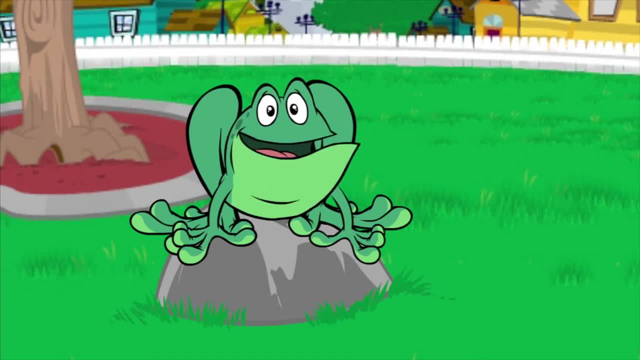 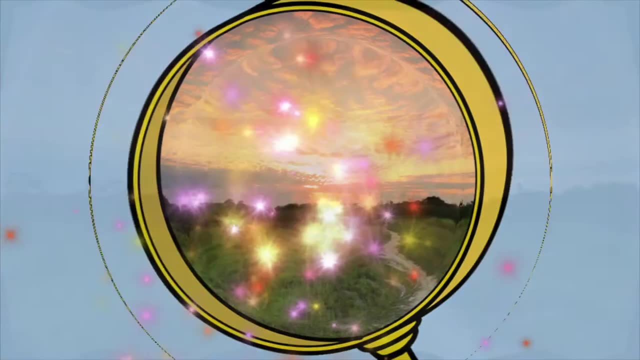 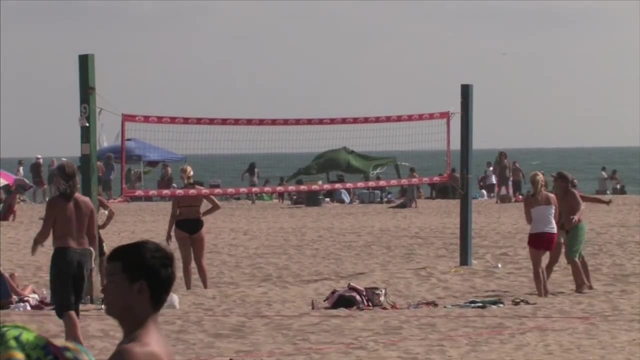 How come, Good question, Do you know why, As the earth spins, the sun appears to move across the sky? When it's direct, the sun moves up the tube. If it moves directly above you around noontime, it is hotter than at the end of the day, when.